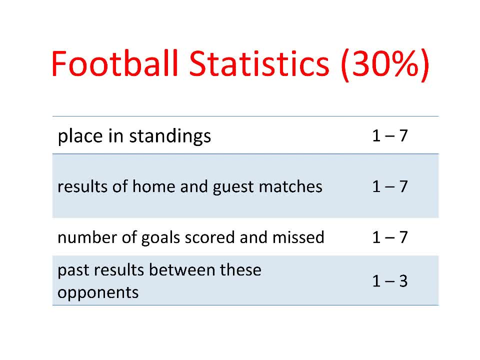 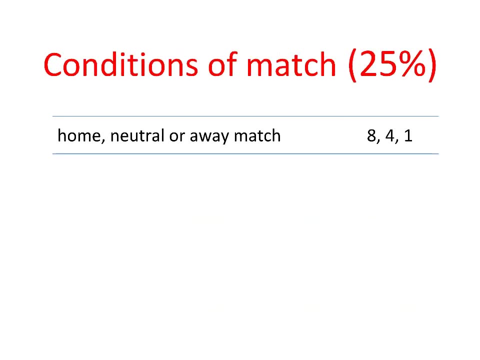 First football statistics Plays in standings: results of home and guest matches, number of goals scored and missed, past results between these opponents. Second conditions: First of all, you need to know the conditions of a match: Home, neutral or away match. 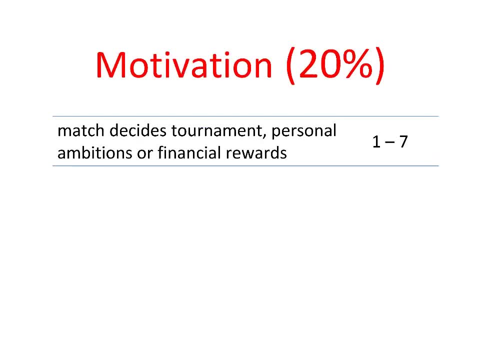 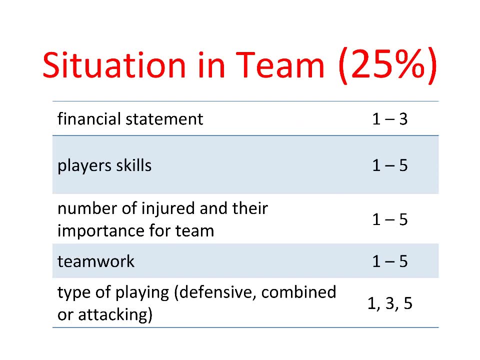 Third, motivation, Whether the match decides tournament, personal ambitions or financial rewards. Fourth situation in team Financial statement: player's skills, number of injured and their importance for team teamwork. type of playing: defensive, combined team. If you look at carefully, you saw near each group symbol of percent and opposite each factor's item figures. 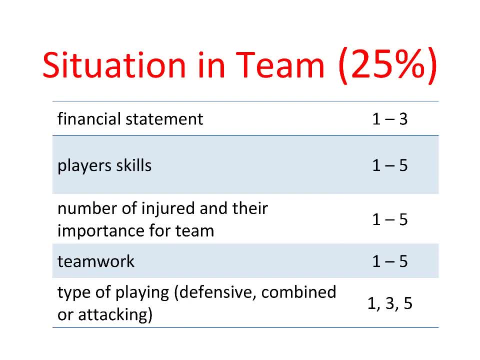 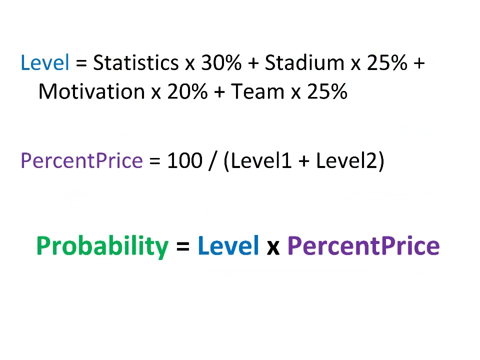 It's very important where dash is range and where comma there is to choose one of opposite options. It's necessary for each of items to put points according to above table Summarize for each factor and put in the formula Level equal Statistics. multiply by 30% plus stadium. multiply by 25% plus motivation. multiply by 20% plus team multiply by 25%. 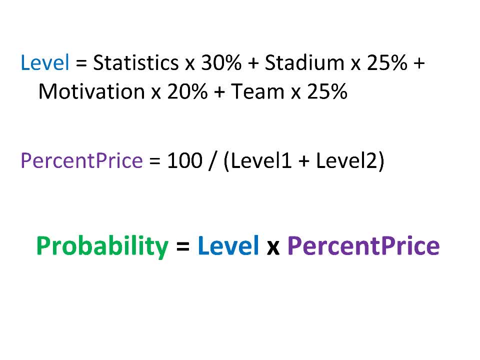 Calculating scores for each of teams You need to deduce the probability in percent. Percent price equal 100 divided level 1 plus level 2.. Probability: equal level. multiply by percent price One. note: The calculated probabilities in percent exclude a draw. 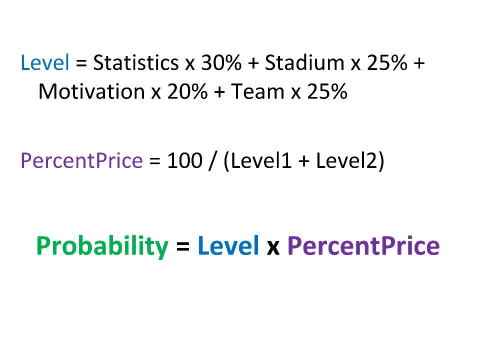 There are odds with handicap 0 for each of two teams. In order to effectively use this algorithm, you perfectly need to understand football and conduct an in-depth analysis of upcoming matches in order to adequately set the scores, And then the mathematics will do work for you. 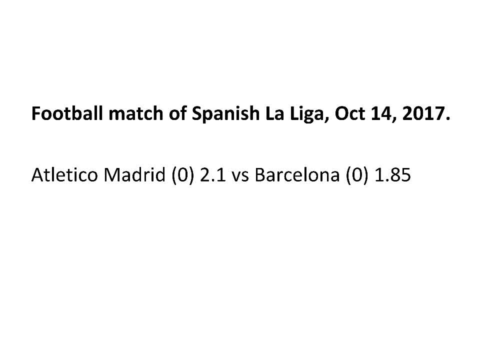 Let's look at an example for clarity. A note: I won't dig into details. I briefly put points on basis of above algorithm Football match of Spanish La Liga, October 14, 2017.. Atletico Madrid vs Barcelona. 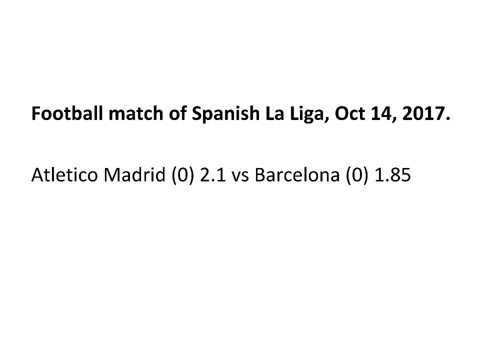 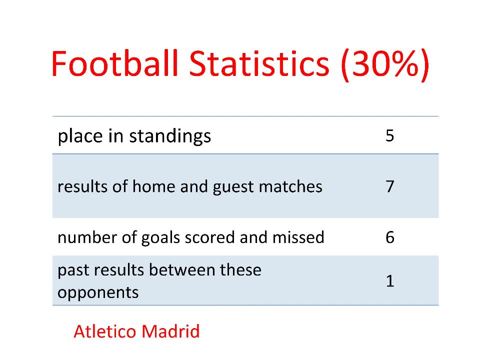 Let's put points for Atletico Madrid. This team plays on own stadium. First football statistics. Position in standings – 5 points. Team takes 5th place and scored 15 points On own stadium. the team played only 2 matches and both won. 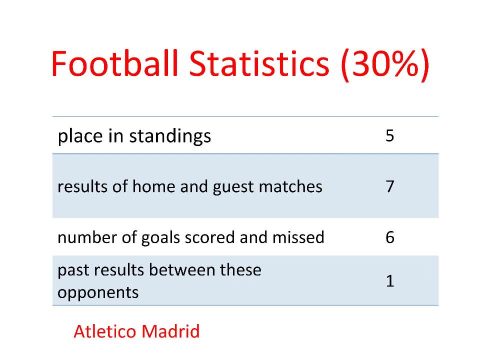 General: Atletico plays perfectly. in its field: 7 points. Number of scored and missed goals: 12 to 4.. Atletico gets 6 points In personal matches against Barcelona team receives 1 point. We will not take the whole history. 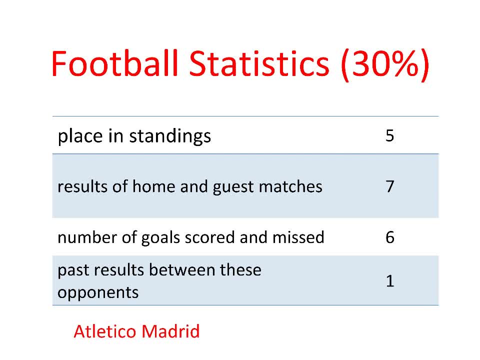 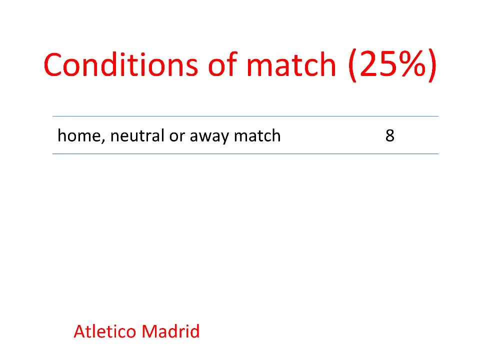 For the last 5 years, only 17 matches Have won: 3, 6 draws and 8 lost Totally. according to statistics, Atletico scored 19 points. Second for own stadium, Atletico gets 8 points. 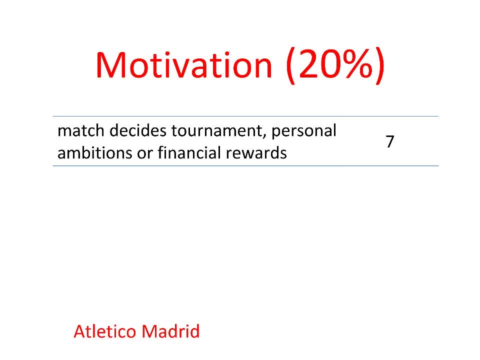 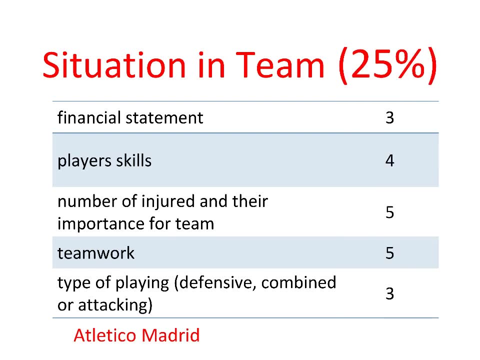 Third match is important for Atletico: 7 points. The situation in team Financial statement: 3 points. Skill level of players: 4 points. Almost no injured and players ready for the match: 5 points. Players are perfectly coordinated, which is other. 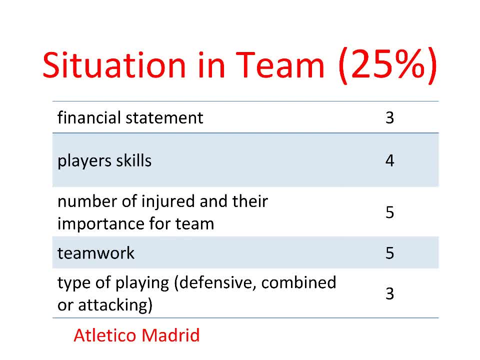 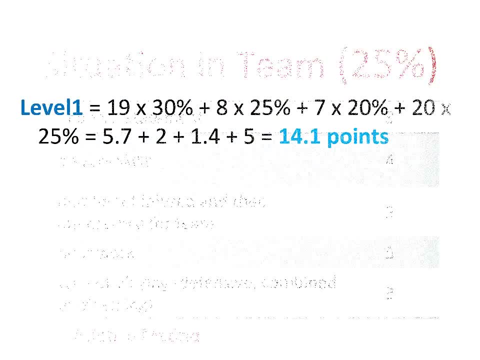 5 points. Combined team playing style: 3 points. Total for the situation in team: 20 points. Let's add all points for Atletico Madrid In above formula: Level equal: 19 x 30%. 8 x 25%. 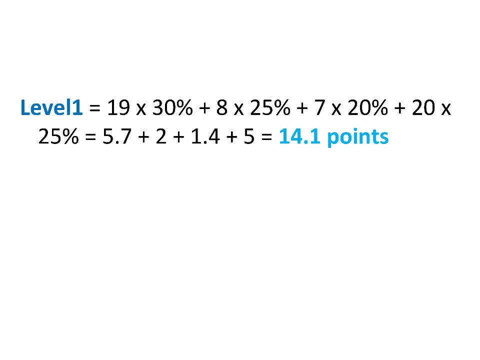 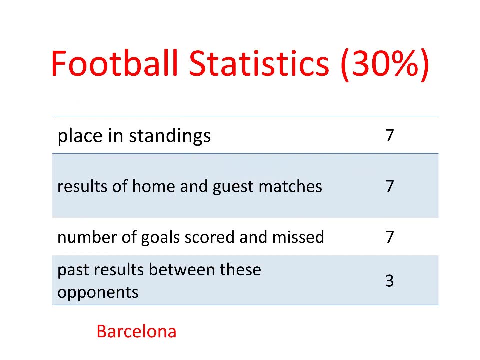 7 x 20%, 20 x 25%, We get 14.1 points. Now let's calculate for Barcelona First football statistics Position in standings: 7 points: Team takes first place and scored 21 points of 21 possible. 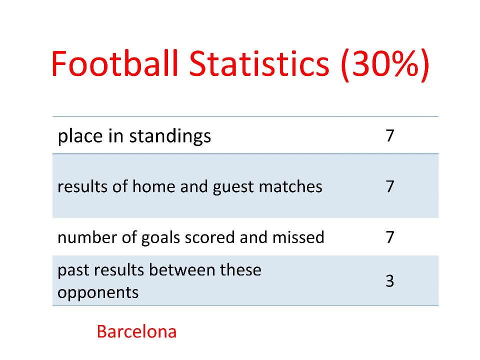 Away. Barcelona played 3 matches and won them 7 points. Number of scored and missed goals: 23 to 2.. 7 points. Personal matches against Atletico: Team receives 3 points. Won 8 matches, 6 draw and 3 lost. 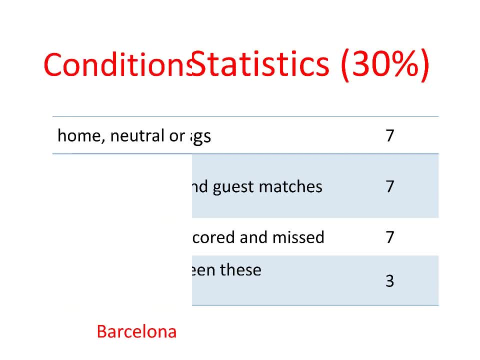 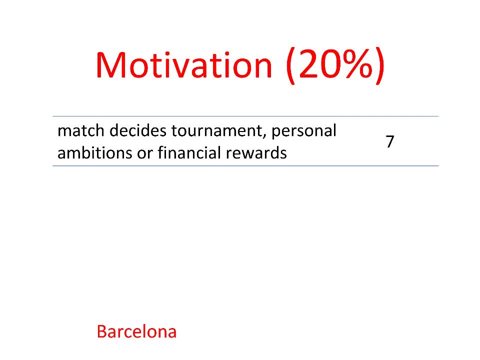 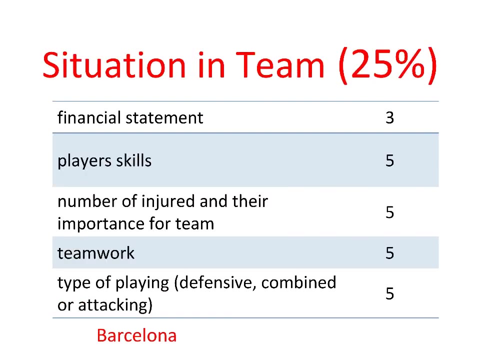 Total. for statistics: Barcelona get 24 points. Second Away match for Barcelona: 1 point 3.. The match is important for Barcelona in order to keep first place: 7 points. Fourth, Situation in team Financial statement: 3 points. 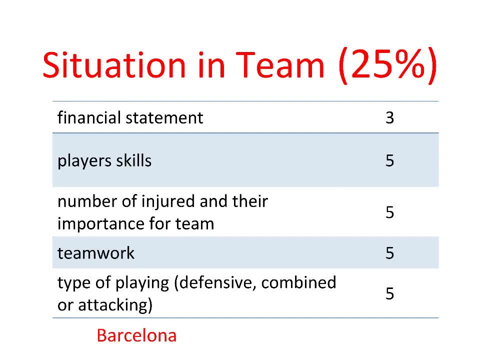 Skills level of players: 5 points. Almost no injured and players are ready for match. 5 points: Players are perfectly played among themselves. 5 points: Attacking style of Barcelona playing. 5 points Total for situation in Barcelona. 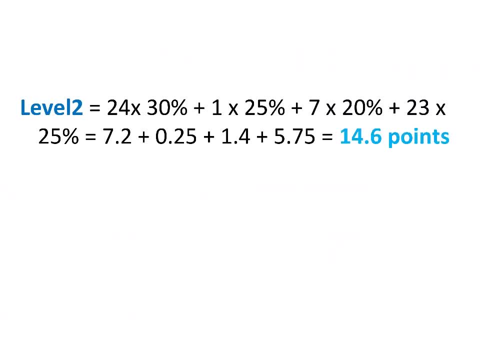 23 points. We substitute the obtaining data for Barcelona in the formula Level equal 24 multiply by 30% plus 1 multiply by 25% plus 7 multiply by 20% plus 23, multiply by 25%, And we get 14.6 points. 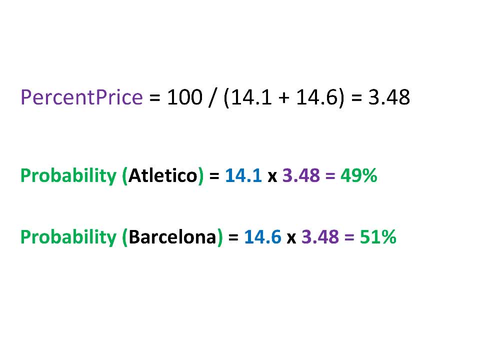 Now let's calculate pass and price. Pass and price equal 100 divided 14.1 plus 14.6.. We get 3.48.. Atletico probability: 14.1 multiply by 3.48.. We get 49%.